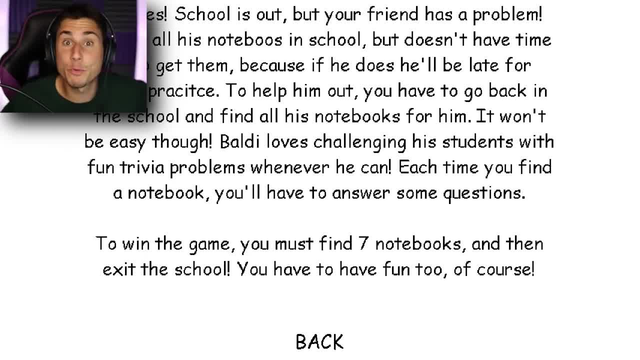 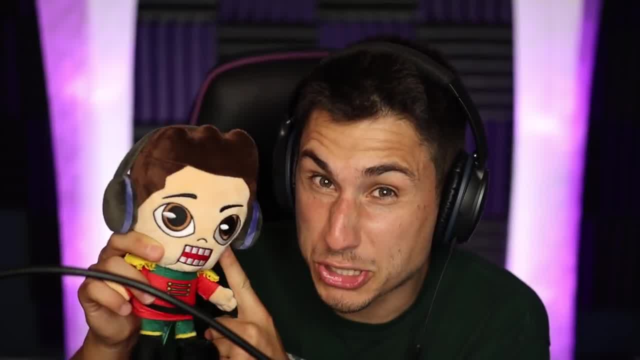 Let's see if there's a story. Nope, there is not. Well, you guys love when I write my own stories, Ah, beautiful. Also, I've mentioned it before, Don't forget to pick up one of the brand new frustrated gamer: plushie dolls. 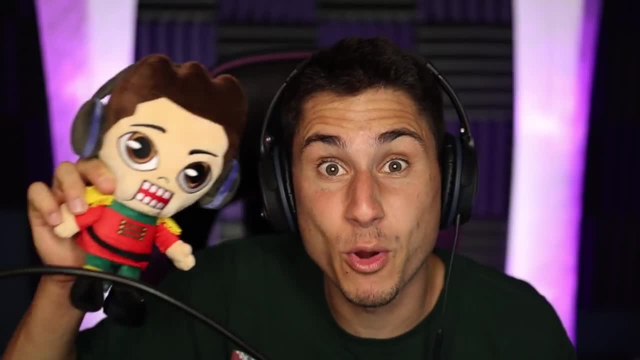 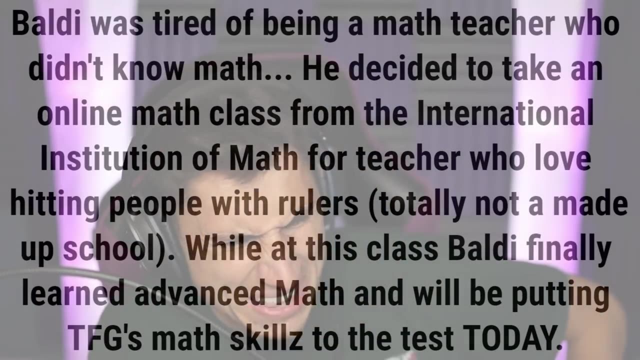 There is a link in the description below. Get it right now, before it runs out. Baldi was tired of being a math teacher who didn't know math. He decided to take an online class from the International Institution of Math for teachers who love hitting people with rulers. 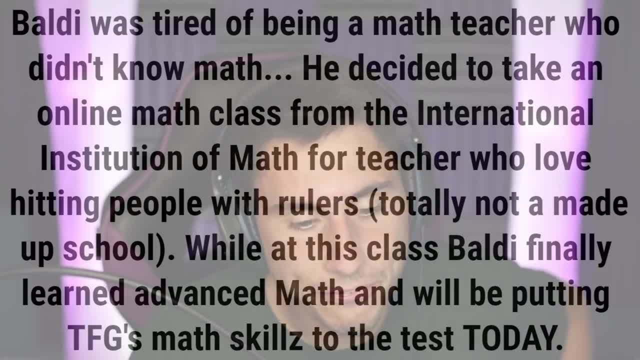 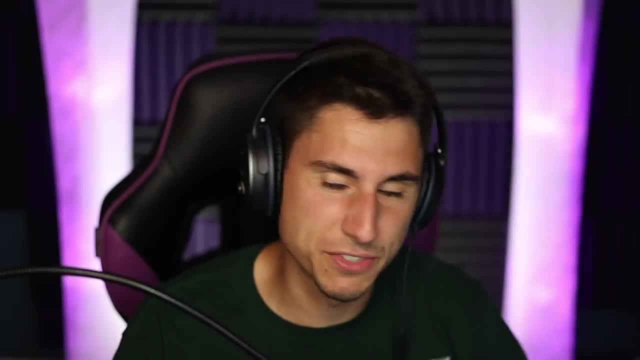 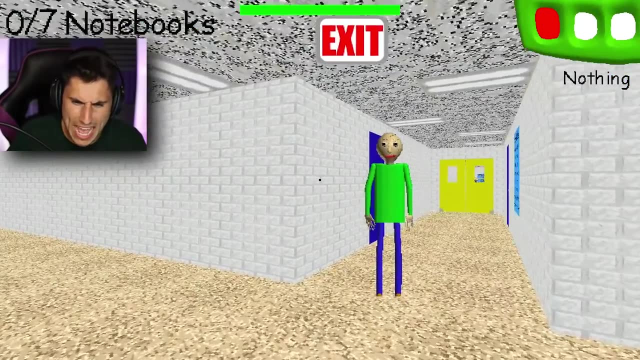 Totally not a made-up school. While at this class, Baldi finally learned advanced math and will be putting TFG's math skills to the test today. Ah, this is just fantastic. Hey Baldi, Welcome to my-. Okay, everything looks very normal right now. 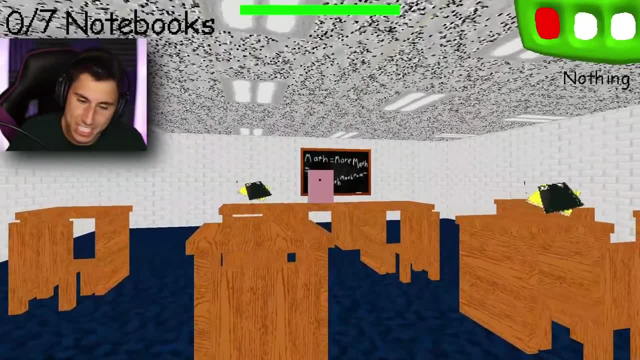 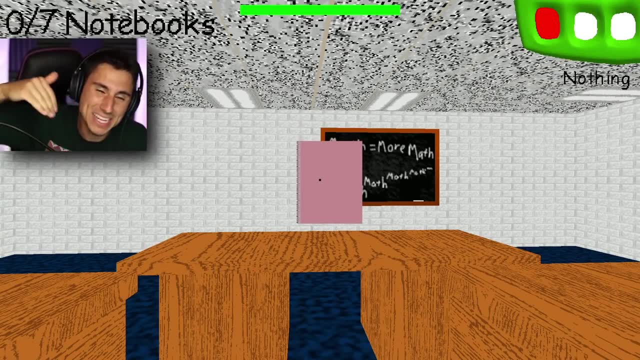 I'm just waiting for the mod to kick in. Someone told me that these math questions are going to be really hard and I'm going to have to use a calculator, which is kind of embarrassing to have to use a calculator in Baldi's basics. 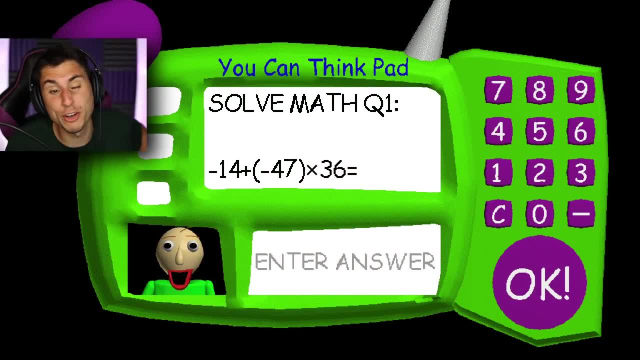 Oh my gosh, Here we go. I got to remember order of operations, So parentheses and then multiplication. Let me take out my phone and try to figure this out. You know what We're going to do. the calculator right here. So you guys see what I'm doing. 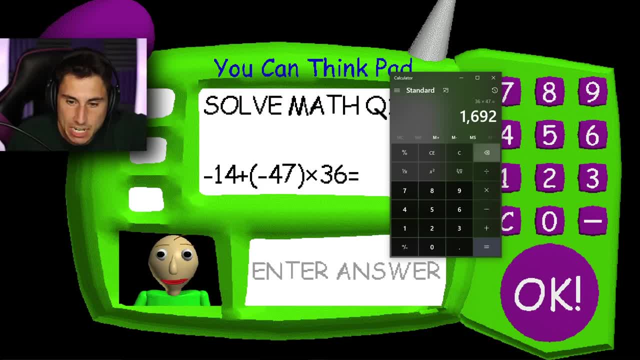 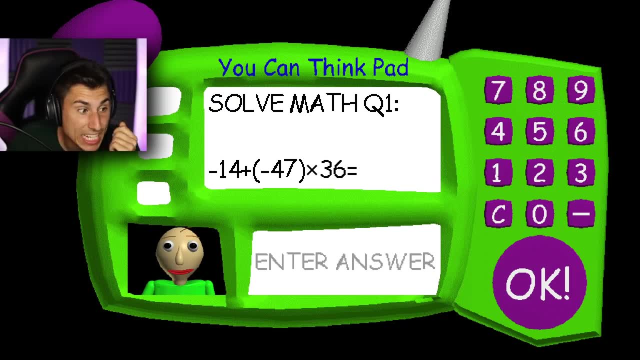 So it's going to be 36 times 47,, but that's going to be a negative number Minus 14.. I'm so confused. I think it's going to be negative 1,678,, but I'm probably wrong. 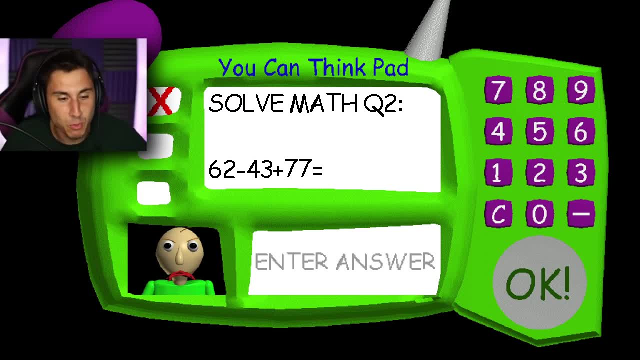 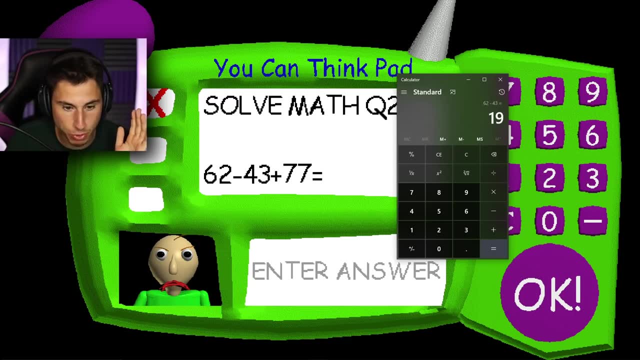 1,678.. Enter The first one. I already got wrong. All right, this one should be a little easier. I'm still going to use a calculator: 62 minus 43 plus 77. If that's not, 97,. 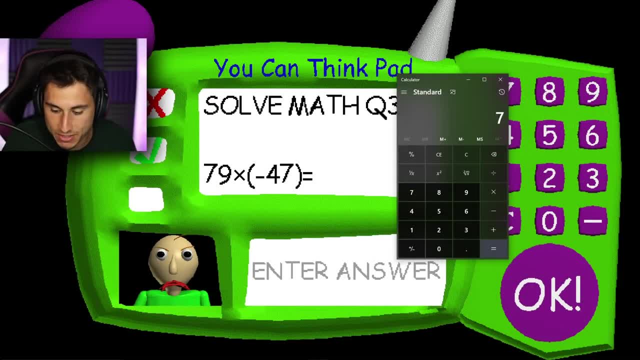 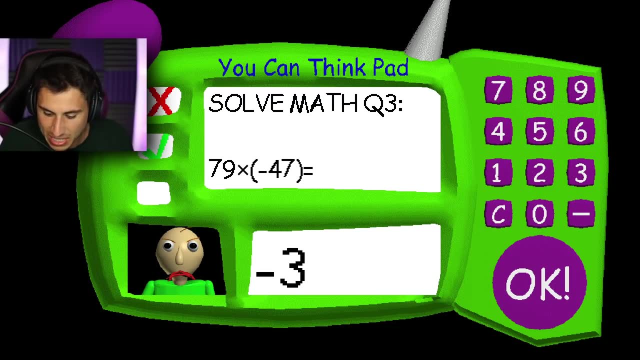 I'm going to smack somebody. Okay, this one's going to be 79 times 47, but it's a negative number, So negative 3,713.. Okay, so is Baldi going to get me. He's already coming after me. 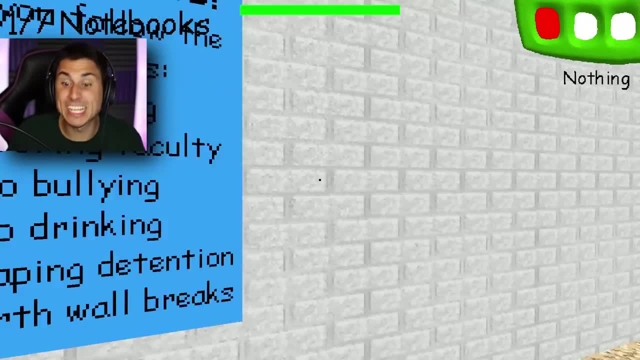 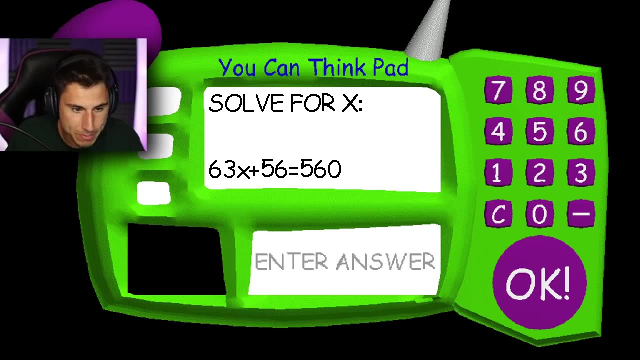 But what was that sound? What? That was a terrifying sound. It sounded like somebody broke Baldi's ruler and then he got angry and went Super Saiyan on me. Okay, here we go again with the wait a second. Solve for X. 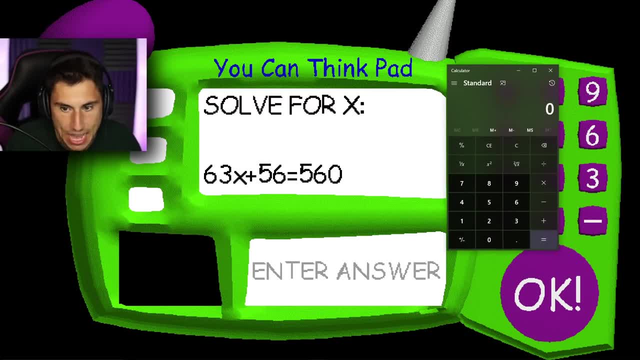 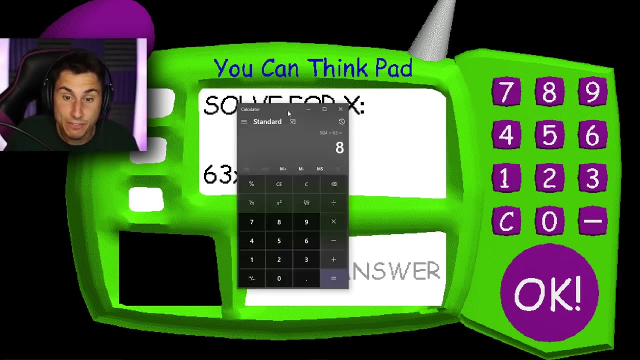 Wait a second. This one should be a little easier, So let's take out our handy-dandy calculator once again. So we're going to do it backwards. 560 minus 56 equals 504. divided by 63 is 8.. If this one's 8, I'm very proud of myself. 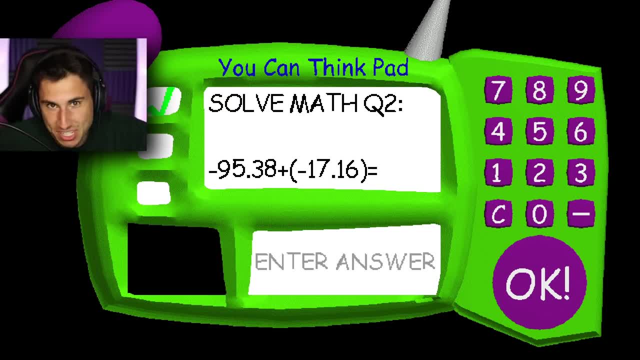 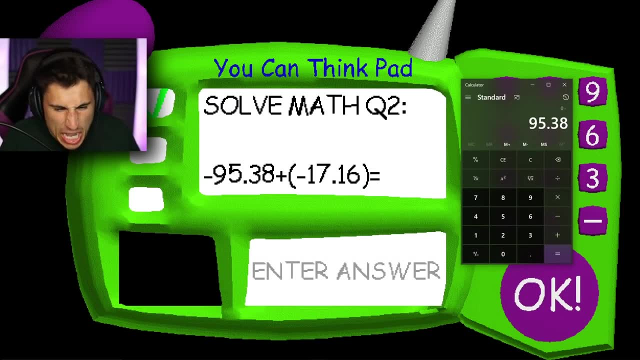 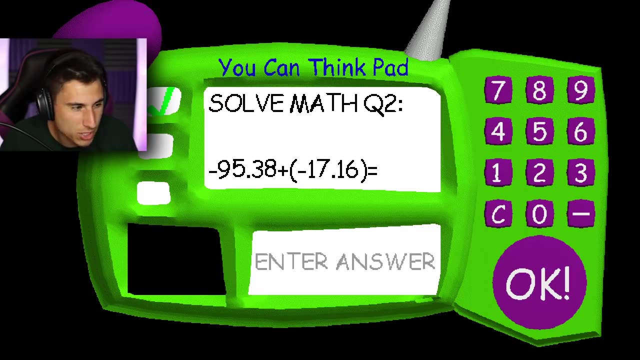 8.. Yeah, all right, You guys are going to have to help me with some of these math questions because there's no chance I get these right. This one: we've got negative 95.38 plus minus, So I think it's just minus 17.16, negative 112.54, 112.54.. 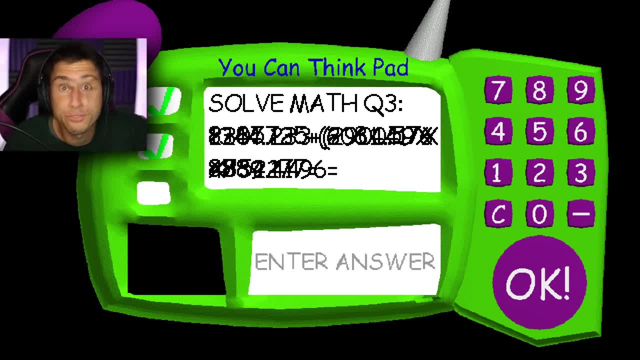 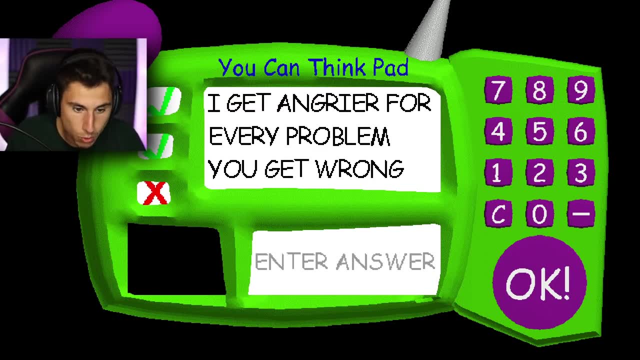 Okay, and as if these math questions weren't already hard enough, Baldi's going to give us the gobbledygook, which I'm just going to put random numbers in. Okay, this is fantastic. I've already gotten two math questions wrong. 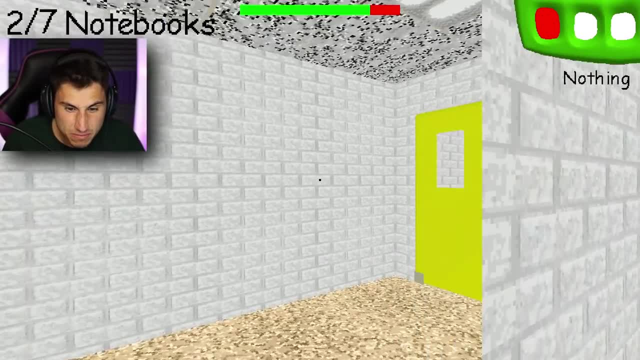 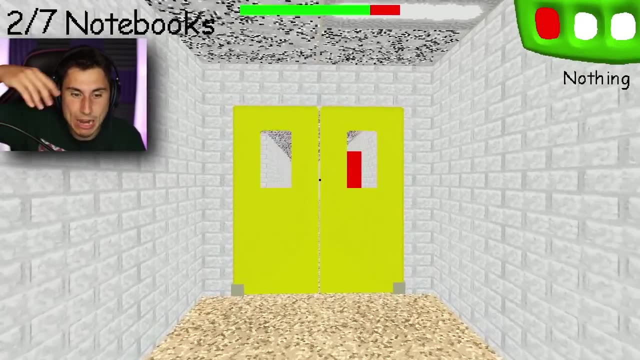 which means Baldi's going to be faster than normal. Okay, I don't hear Baldi yet. Did he explode in the beginning of the mod when there was that really loud sound? Maybe? Nope, now I hear him Darn it. 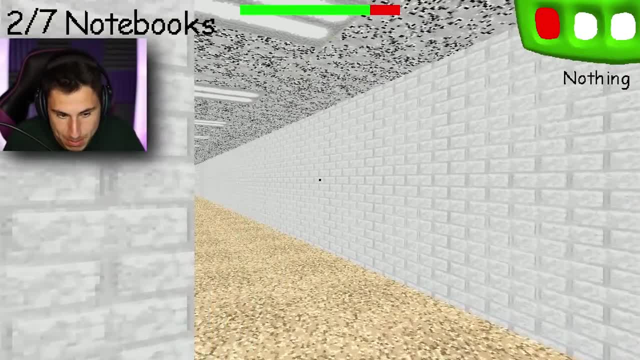 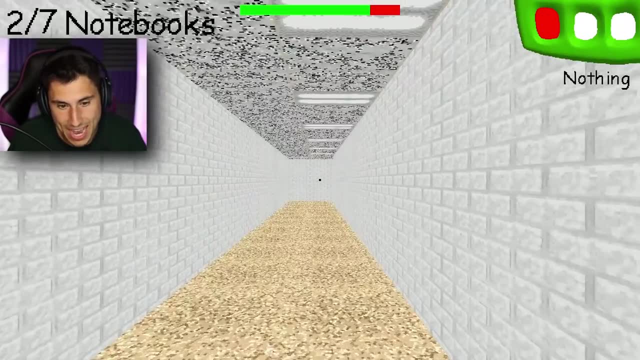 I was really hoping. maybe Baldi spontaneously combusted, or maybe his his ruler exploded and accidentally killed him, I don't know. Okay, Baldi sounds like he's fast already. This is not good. All right, let's go in here. 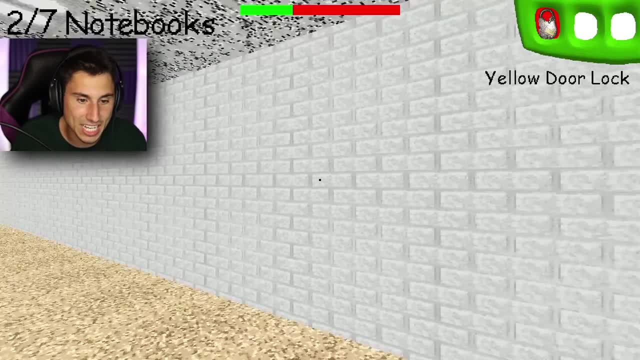 Hopefully we don't get a detention. I also didn't get a shiny quarter because I got the first one. No entering school faculty, only rooms in the hall. You've got to be kidding me. You've got to be kidding me. 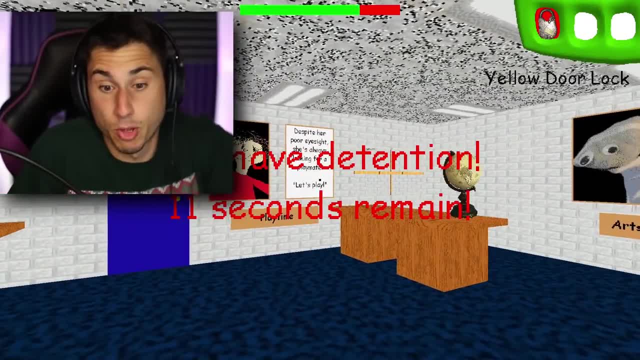 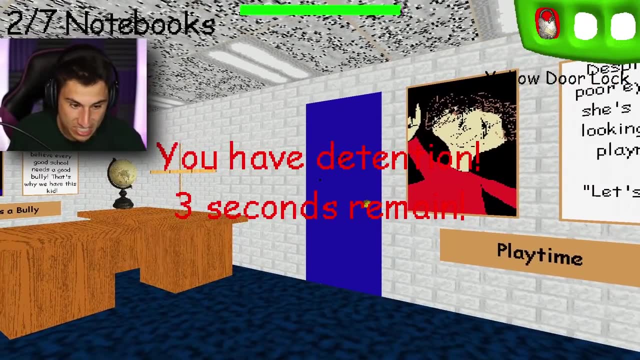 At least there was a shiny quarter at the end of the hallway And then the principal came here and ruined everything. Where's Baldi? All right, we got eight seconds. Come on. I know this is advanced math. It's not advanced time. 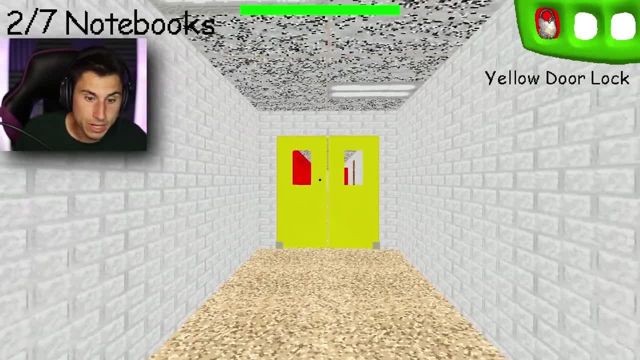 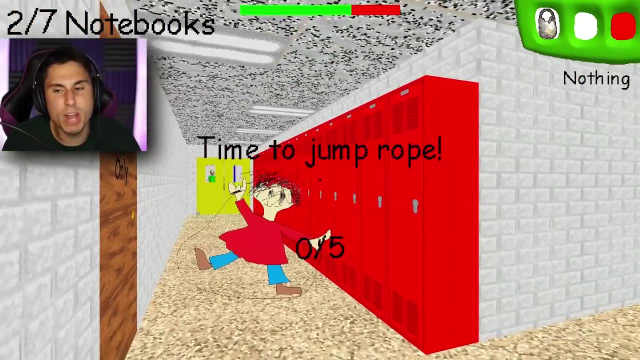 Let's keep going. Let's go this way. He's that way. Wait, is he? No, no, no, we can't play. We can't play. No, playtime, playtime, No, no, playtime, playtime. 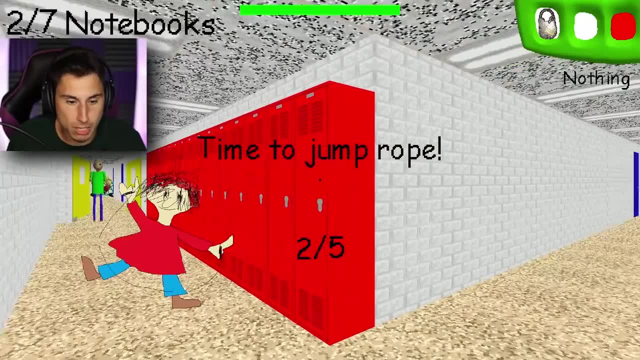 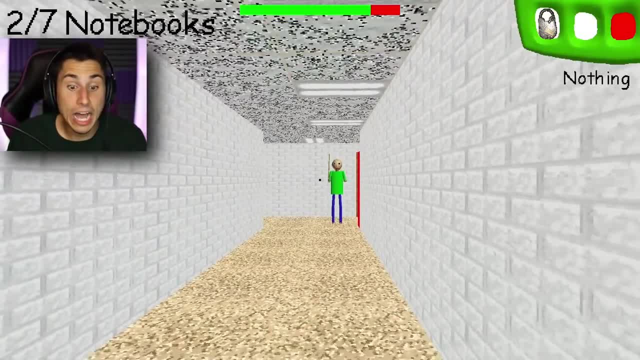 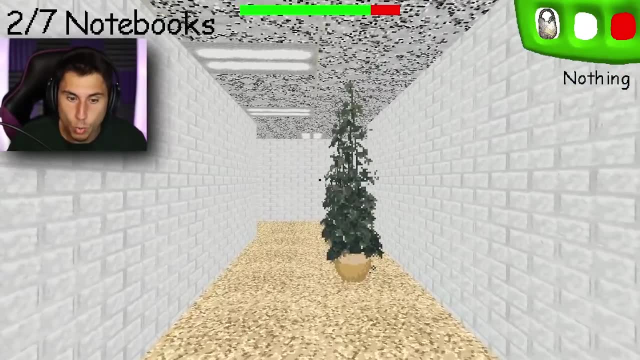 Come on, come on, come on Run. Okay, I cannot believe I somehow got away from Baldi there. Okay, I have a plan. It's not a good plan, but it's a plan. We're going to go all the way around. 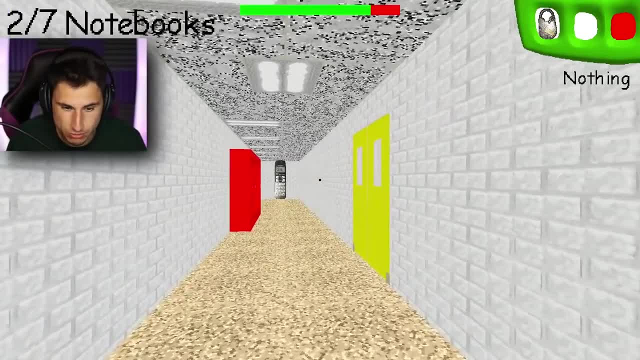 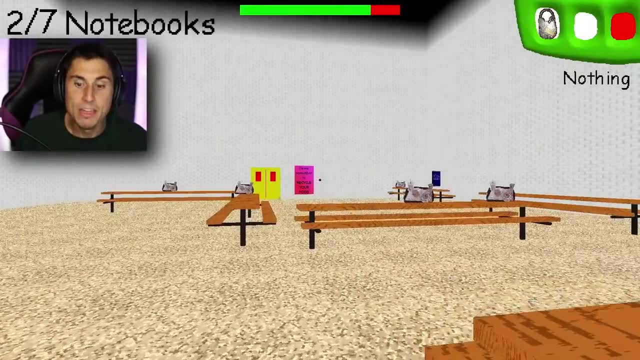 Baldi is slower than me so far because I only got two math questions right or two notebooks right so far, which is kind of embarrassing. So let's grab this bee soda right here on our way, Then I'm going to go down that really long hallway. 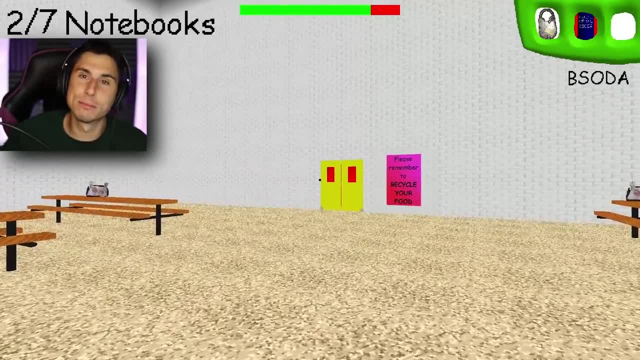 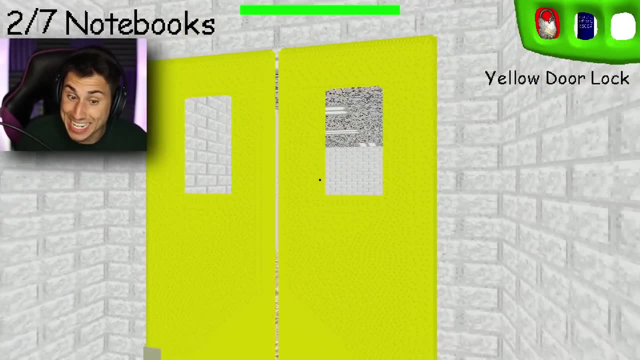 but I'm going to use the yellow door line. I don't even know what I'm talking about, but you guys are going to have to just kind of watch and see what I do. And there is another shiny quarter right there. I'm going to wait for Baldi to catch up to me. 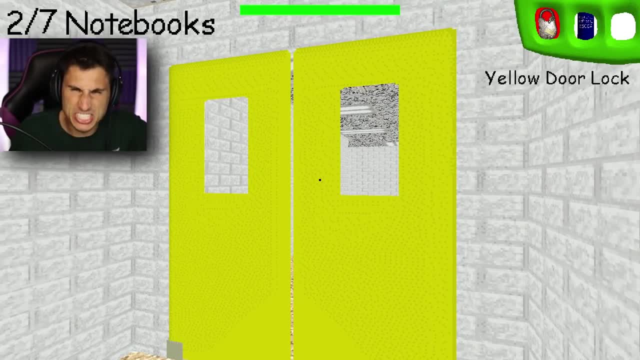 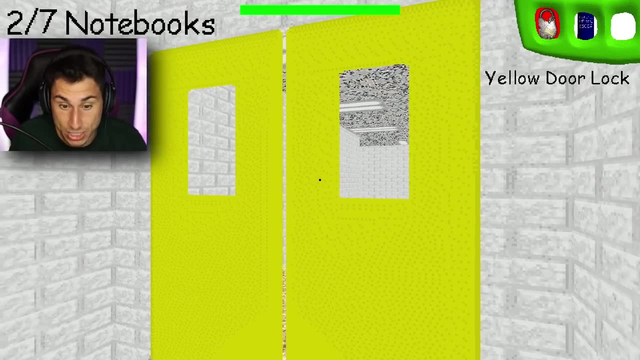 And then I'm going to use the yellow door lock here. So this is kind of like the same door. I normally use the door lock, but on the other side, if any of this is making sense, this is: this is way too advanced for me. 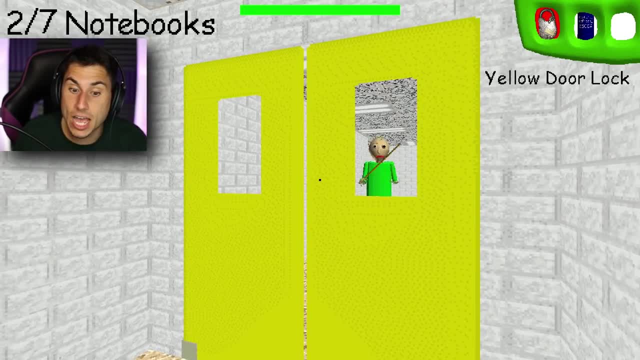 Okay. so here comes Baldi. I'm going to wait for him to move one more time and then bam. Okay, so he's going to have to go all the way back around. I'm going to grab this shiny quarter. And now the bully is there. 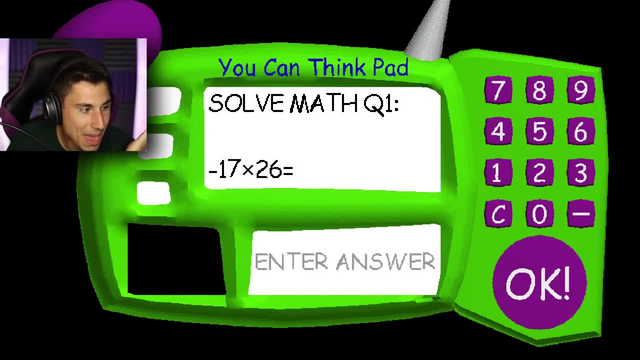 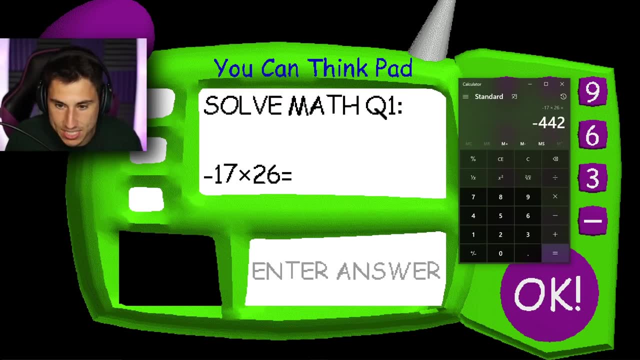 Let's do. I forgot the math questions are hard. I literally forgot the math questions are hard, even though that's the point of this entire mod. So we got negative 17 times 26.. That's negative 422.. Honestly, that one was pretty eat. 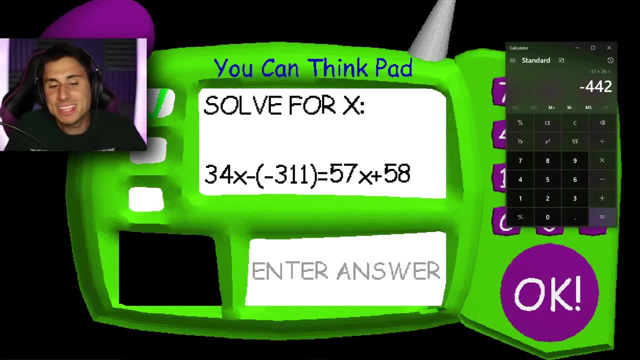 Oh my gosh, What is this nonsense? I mean, this might as well just be gobbledygook. at this point, I'm going to use my brain and try to figure this one out Three weeks later. This one has taken me a very long time. 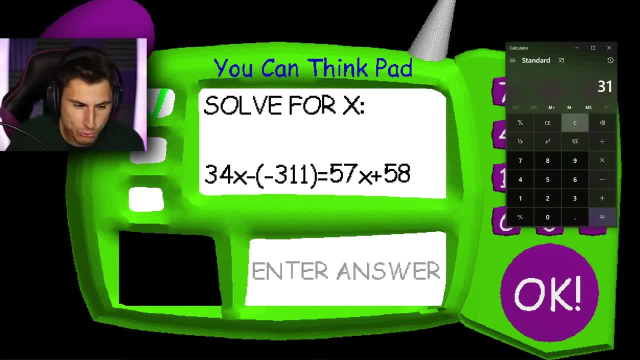 And I still probably have it wrong. So this is the point that I'm at: 311 minus 58. So that's 253 equals 23 X. I am 100% wrong here. So we're going to divide that by 23.. 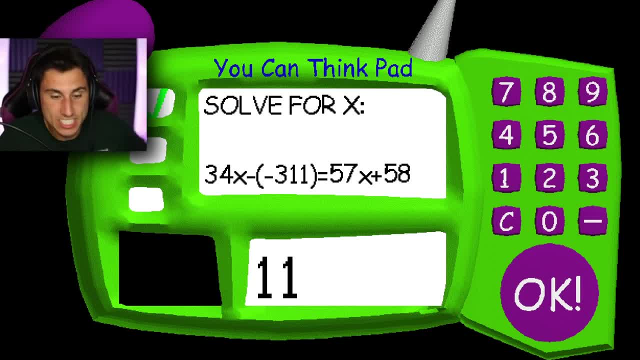 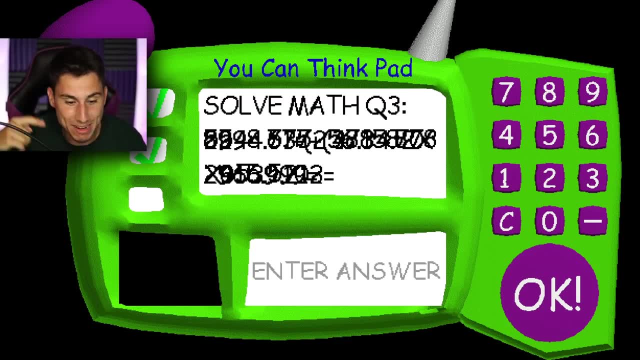 Maybe it's 11.. If this is 11, I am going to dance around this entire room screaming: I am very proud of myself, even though that's like sixth grade Math. I've been out of sixth grade for a long time, guys. 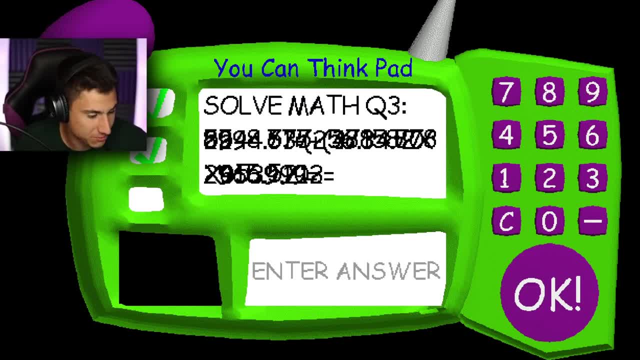 Okay, Yeah, I have like notes all over my desk from this mod. so far, Okay, And now we've got gobbledygook. We're going to go here. It is 78,944.. If I was able to get that last one. 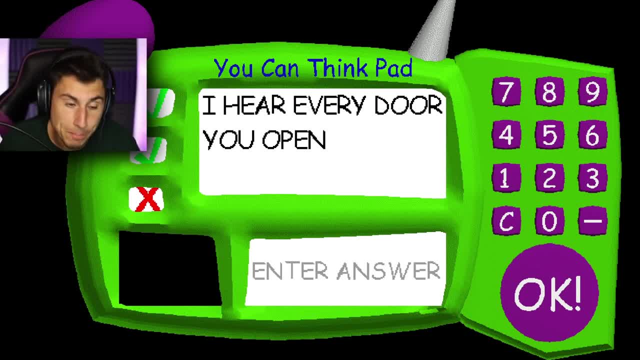 I feel like I could get this one. Nope, All right, that one kind of burst my bubble a little bit. At least I got the one. Okay, I I have been in the you can think pad for so long, I don't even remember where I am anymore. 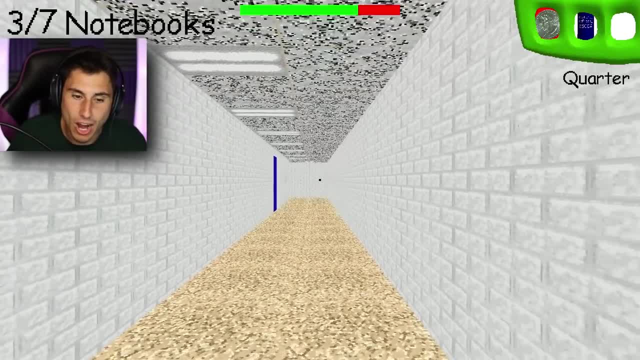 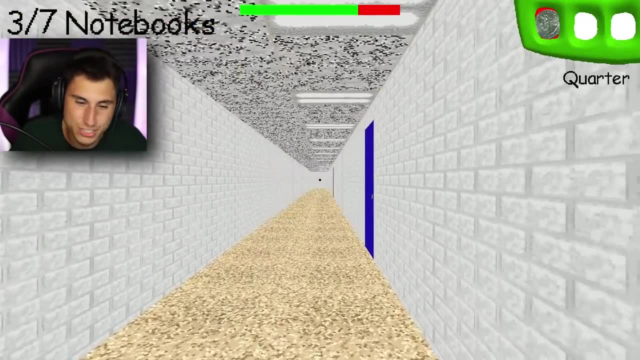 Is the bully behind. now He's in front of it. All right, I got a prey that he takes the shiny quarter. I guess it really doesn't matter. He took the B soda. He took the B, said. of course he took the B soda. 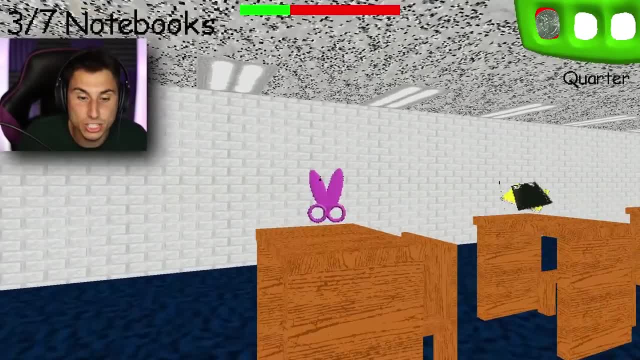 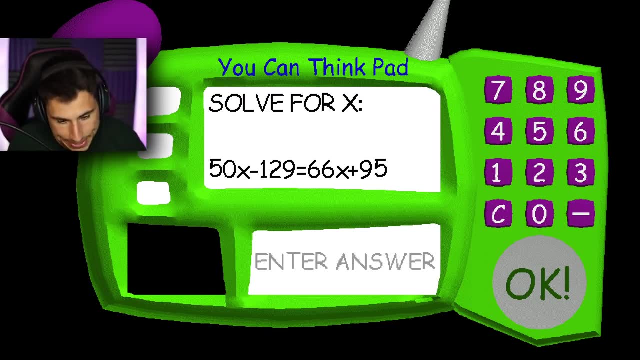 Why wouldn't he take the B soda? This mod is just designed to torture me. Okay, I got that, And now this one's another one. Oh my gosh, Let me take out my notepad again. Negative 129.. Get rid of the 50 and make the X of 16 plus 95. 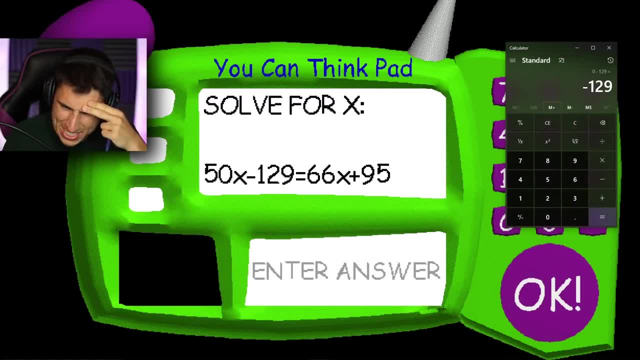 So I subtract the 95. Negative 129 minus playtime. Will you shut up? I am trying to do a math question right now. Oh my gosh, She's driving me nuts. I think it's negative 14.. Come on. 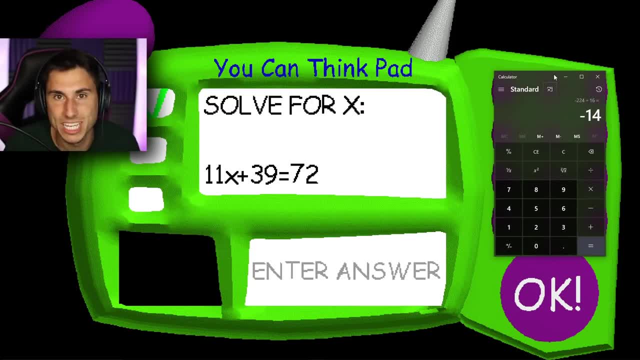 Whoa. Okay, Now I'm proud of myself. Now I'm getting overconfident. I'm probably going to mess up like 4 plus 4 at this point, Okay. So this is how I'm going to do it. 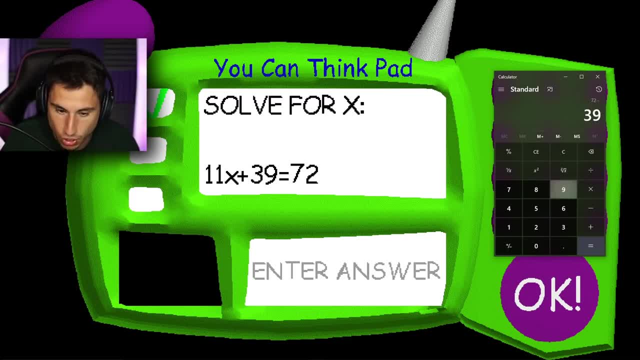 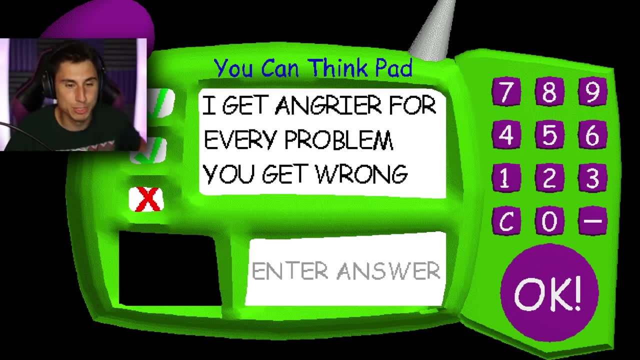 You subtract the 39 from both sides, That's 72 minus 39. So we've got: this one's going to be three. This one's just three, Yes, and then we've got gobbledygook. Okay, I am brushing up on my algebra. 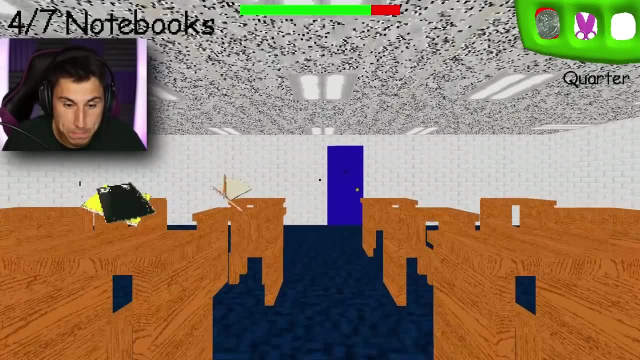 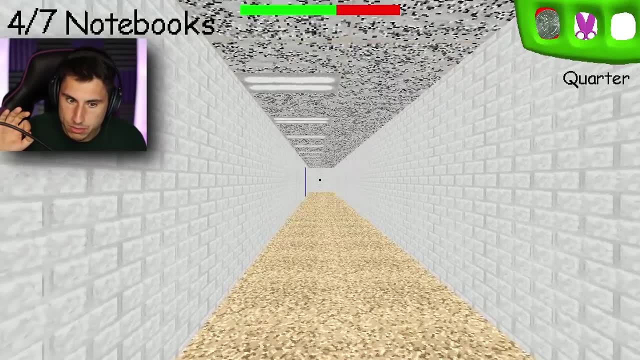 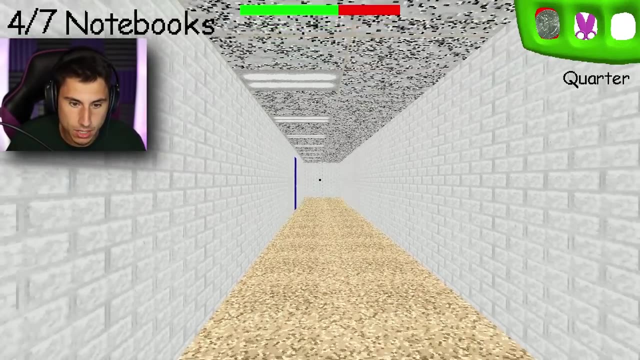 My? I don't even remember who my algebra teacher was. I think his name was Mr Ockenhouse. Mr Ockenhouse would be very proud of me right now. Okay, I'm going to go Where's Baldy? Baldy should be behind me, because I use that yellow door. lock me if I'm walking right towards Baldy. 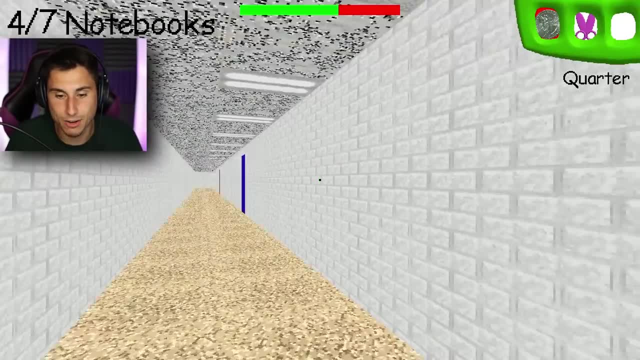 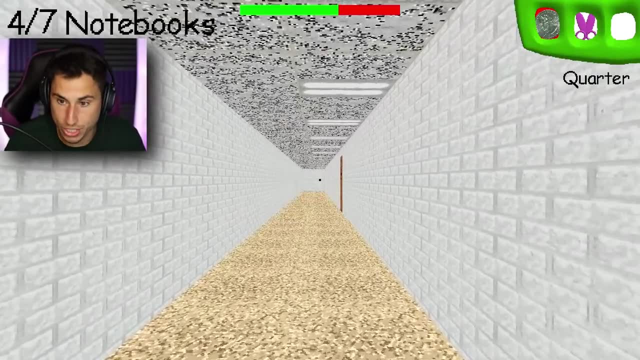 I think I'm running. I don't have to be soda anymore. He's right there. I was walking right towards him. I could have been going up and around the whole time. now I don't have a B soda because Freaking bully took it from me. 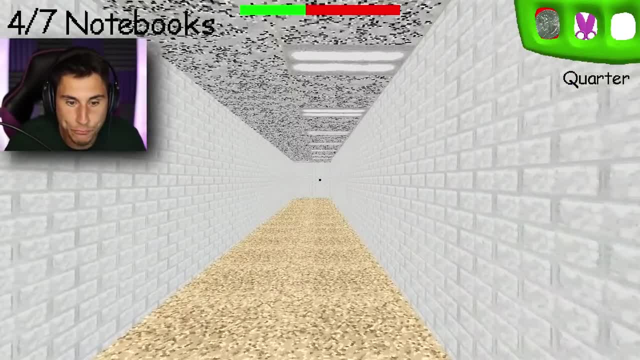 I don't even know what he does with all these B sodas. probably drinks them and that's why he's so fat. Oh, and now I've got a deal with first prize- wanting to give me a hug, Are you kidding me? first price. 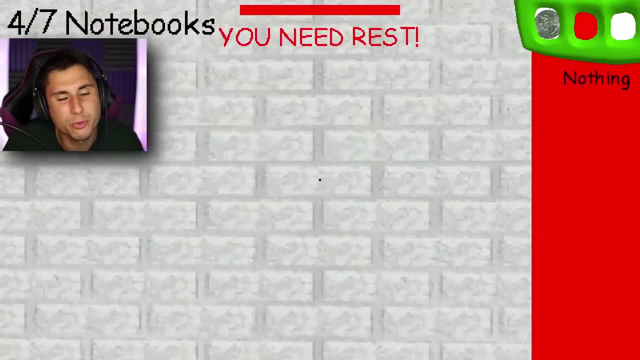 No, I don't want to marry you. I don't want to give you a hug, I don't want to do anything. No, no, no, no, no, No. I won't marry you. I've denied your hand in marriage multiple times. 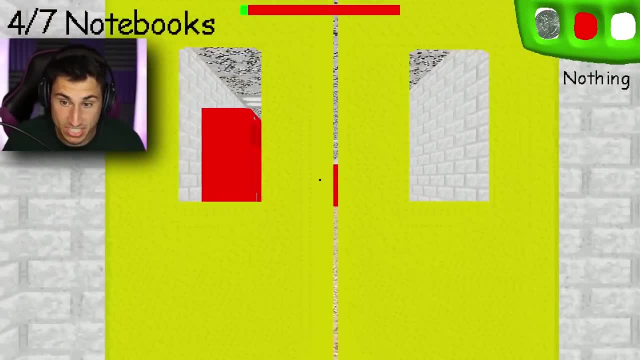 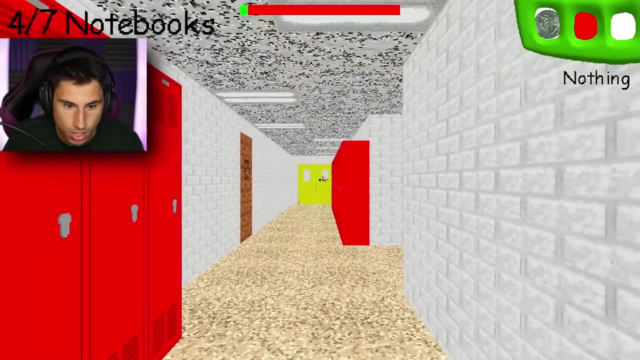 Sam has already agreed to marry me. Okay, this is going to be a race. This is going to be an app. Wait, where's Baldy? Am I going right towards them? No, there's the principal. Oh, Baldi's behind me. but that's okay, because I should be able to get to the vending machine in this in time. 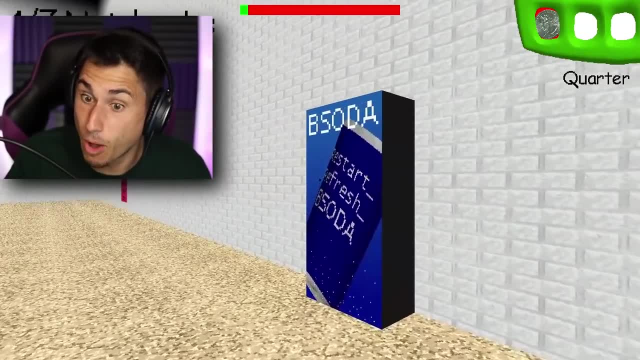 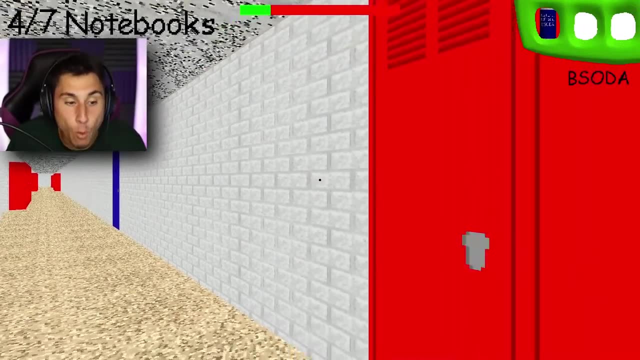 There's a zesty bar over there, and energy flavored zesty bar, So if I can somehow make it down the hallway. I only have four notebooks so far, By the way, I literally only have four notebooks at this point. This is embarrassing. 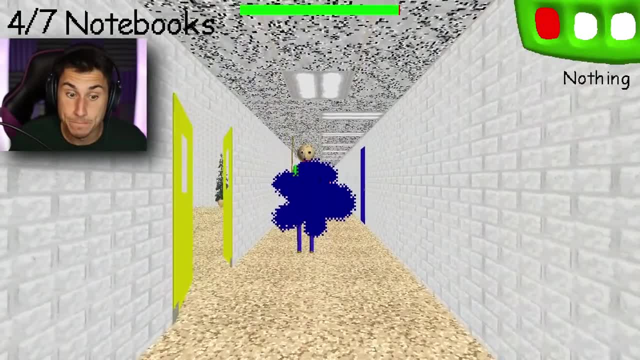 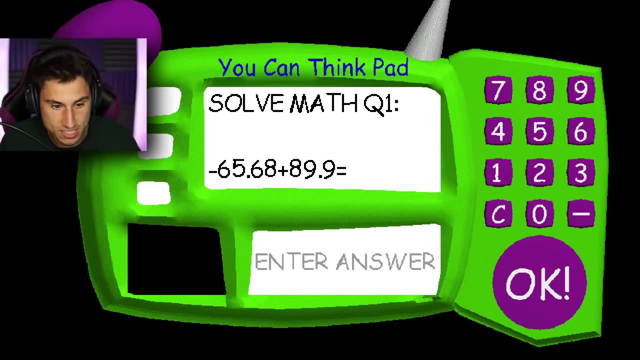 Don't you hit me arts and crafters and hi-yah, Okay, Baldi's going down the hallway. I'm going to grab this notebook. Might as well Get the big old boots, in case first prize decides to bother me. What is this nonsense? 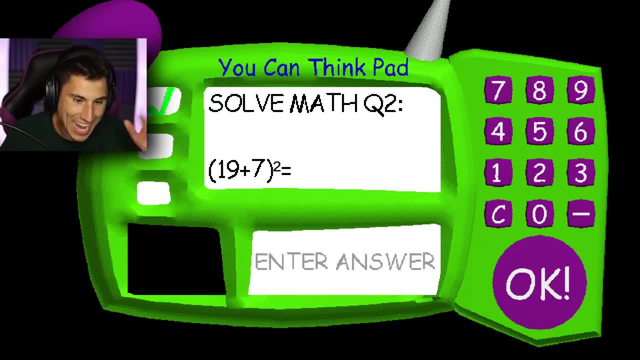 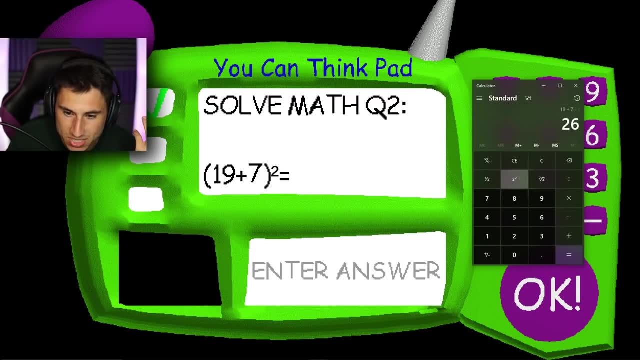 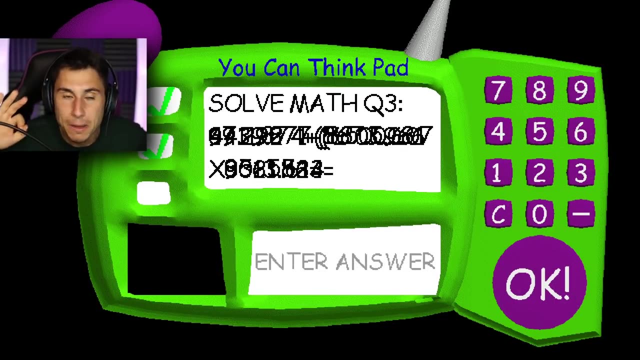 Oh, this one's actually simple, A nice easy 24.22 get out of here. Oh, no parentheses first, So 19 plus 7 to the second power. I think this button, second power, is it 676, 676.. I am so proud of myself today. 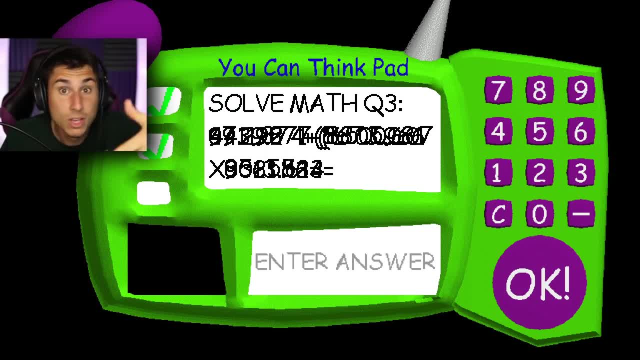 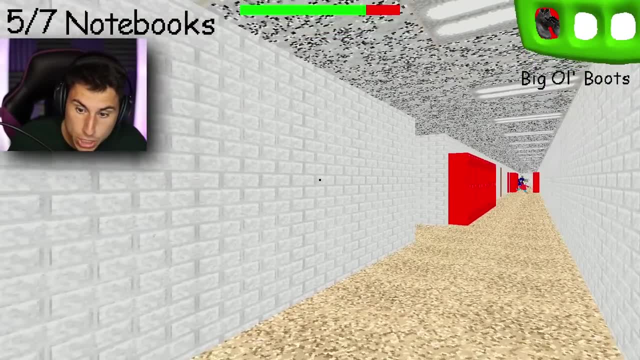 Like I said, Mr Ockenhouse, if you are somehow still alive and watching my videos, thank you for teaching me this, Because this mod would be going a lot worse. So now let's do this. Baldi should still be going down the hallway. 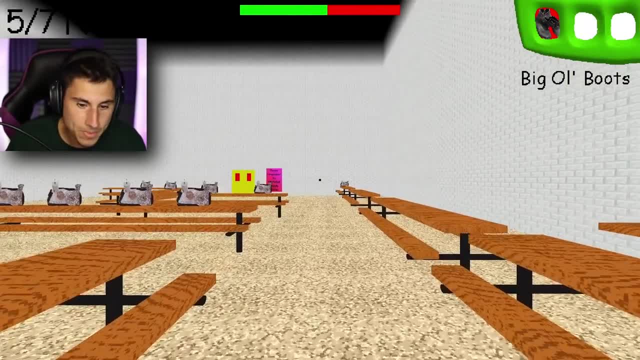 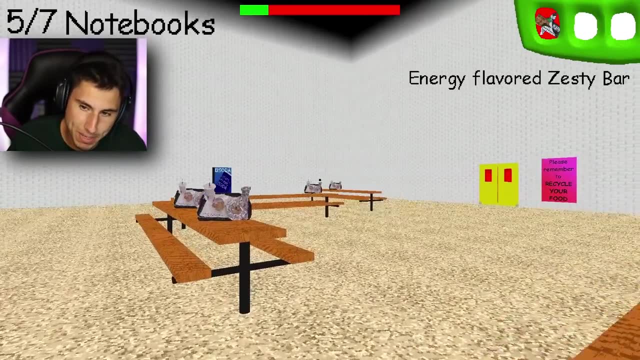 It looks like he is. so we, principal, If you give me a detention. if you give me a detention, I promise I will smack you. Okay, so now we've got the zesty bar, I accidentally use the big old boots. I did not mean to use the big old boots. 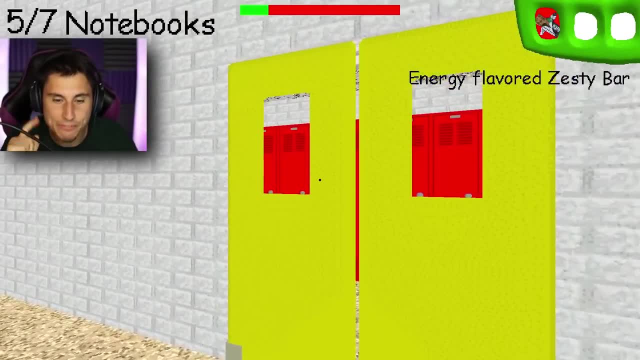 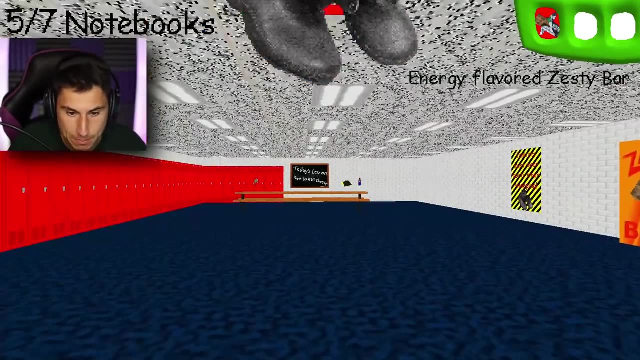 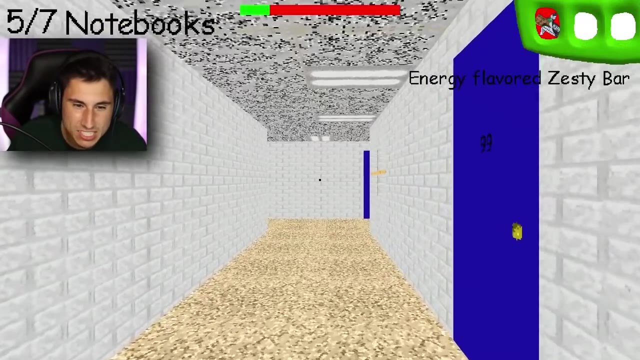 I also really wish I had one more be soda. If I had one more be soda. Okay, I've never seen sweeping time stuck like that before, but I will not argue. There was keys. I need another be soda or maybe even just one zesty bar, even just a zesty bar.